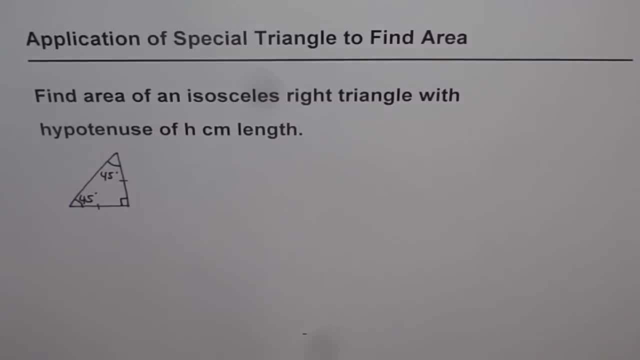 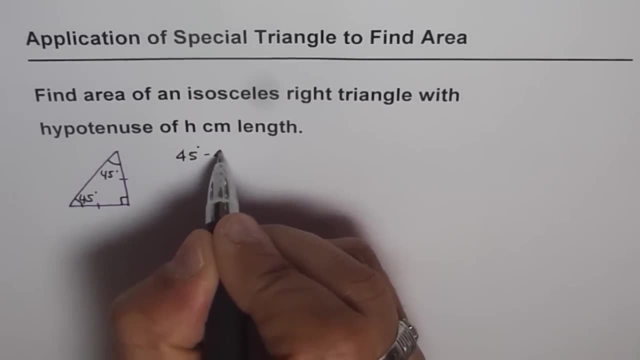 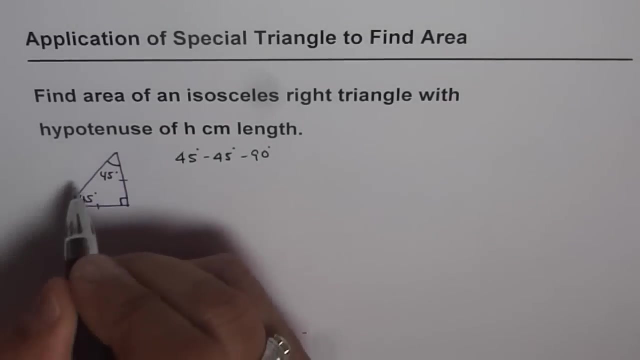 each. So that is how you get your triangle right. So when we have isosceles right triangle, that means we are talking about 45 degrees, 45 degrees, 90 degrees triangle, correct. Now we are given hypotenuse is 8 cm. 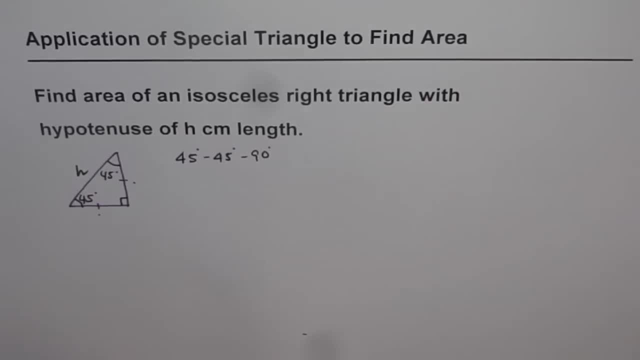 So what is the angle of the isosceles right triangle? So that is the hypotenuse. What are going to be the sides? To find the length of the side, what we can do is we can take help of our standard triangles, which we call special. 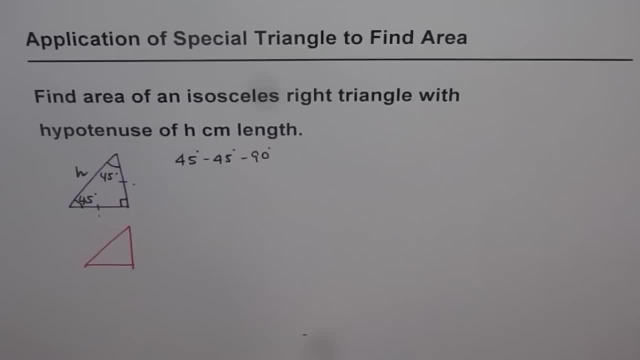 triangles, right. So that is special triangle with sides of 1, 1 unit and hypotenuse of square root- 2 units. Now we have hypotenuse of H. What is going to be the height? This is what we have to figure out. Well, what we can do is we can take help of our standard. 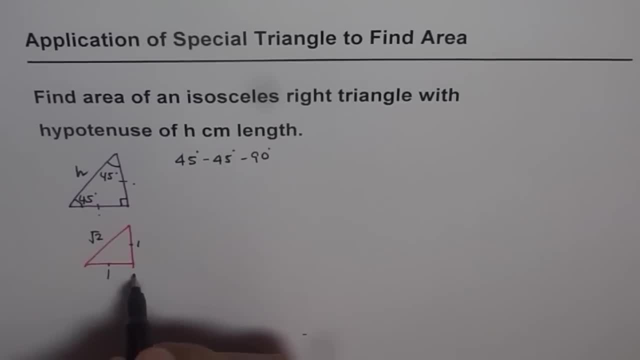 triangles and put them on top of these. So what we have to do is we can put them on top of these and then we are going to put them on top of these, And this is going to be this side of this side. So what we can do is we can further make another similar triangle. 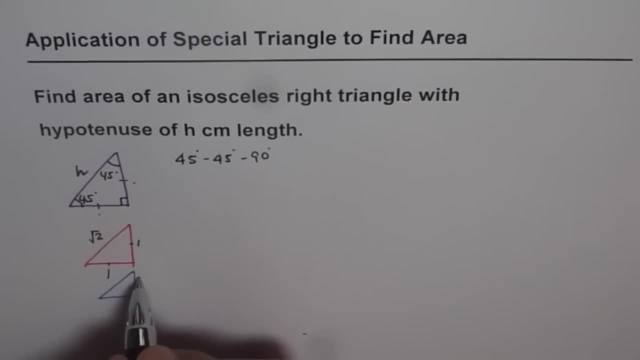 right, Which is 45 degrees, But this time what we will do is we will divide all these dimensions by square root 2.. So what we get here is 1 over square root 2, 1 over square root 2 and this one as 1 over square root 2, sorry, 1.. When you divide square root 2,, 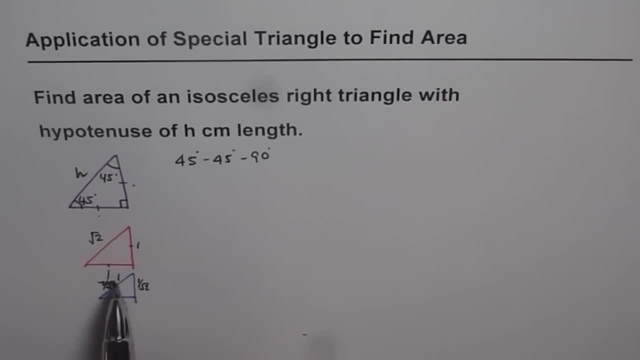 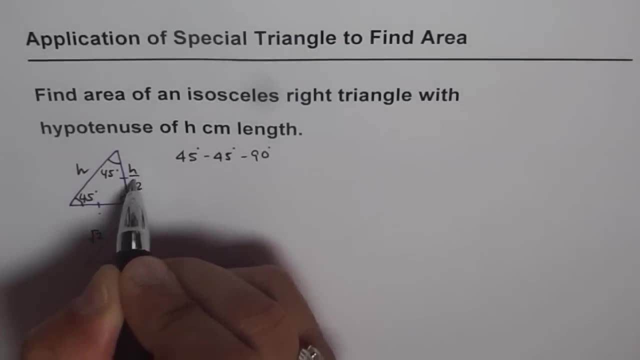 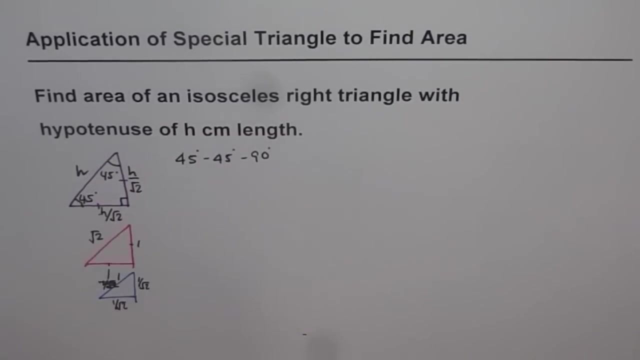 you get 1.. Right, Right, So that is kind of scaling the same thing. Now, if hypotenuse is h, then what should be the height? it's very clear: it should be h over square root 2, perfect. and since height and base are same, base is also h over square root 2. now it is easy to find the 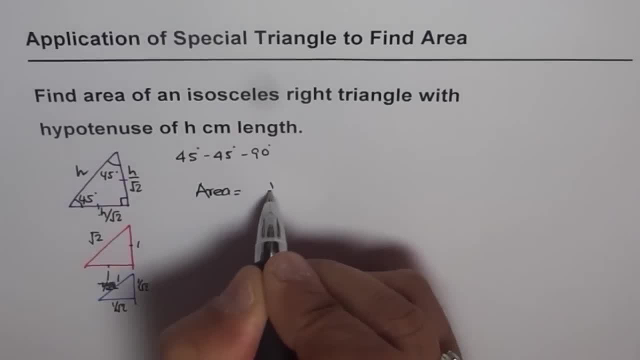 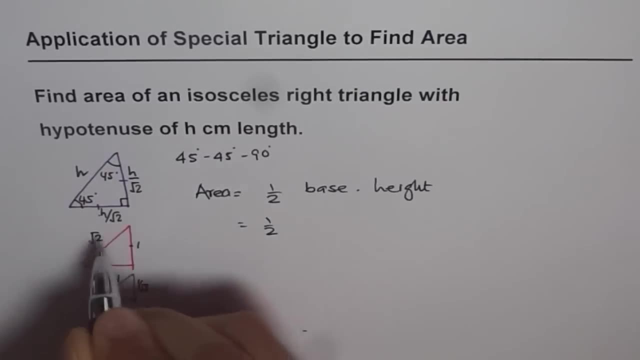 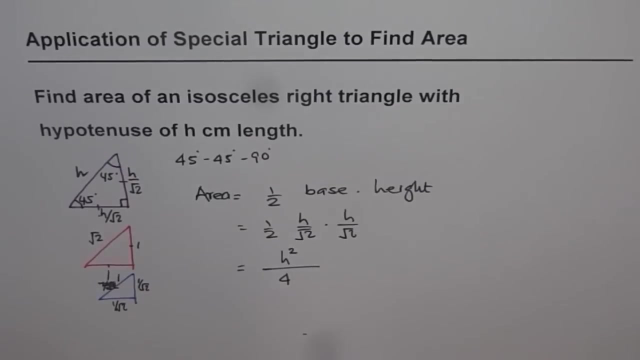 area, right? so the area will be equals to half base times height, which is half of base h over square root 2 times height is also h over square root 2. so what do you get? you get h square over 2 times 2, which is 4, right? so you should remember that area of an isosceles triangle.